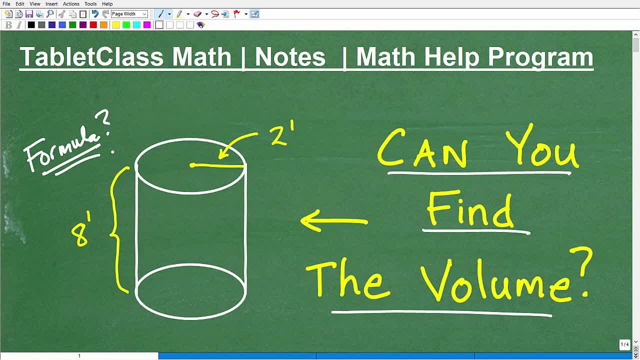 long-term memory. All right, there's a lot of things in math that you know. you just certainly can't remember all this stuff all the time. But basic area and volume and surface area type of formula, Yeah, these are things that you might want to consider. you know, getting into your long-term. 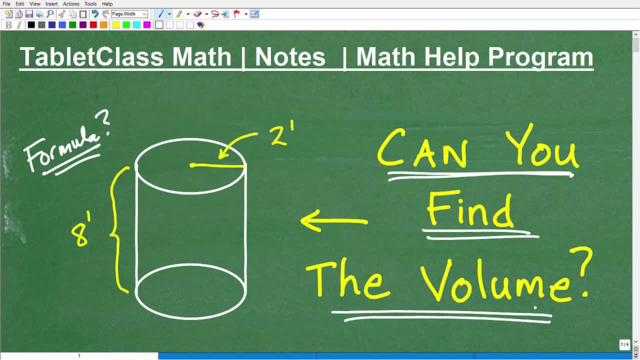 memory And I'll talk to you about how you can do that here in just one second. Now, if you think you could do this problem all on your own, just kind of give you know, turn this into like a little pop quiz for you. Certainly, I would encourage you to pause the video and go ahead. 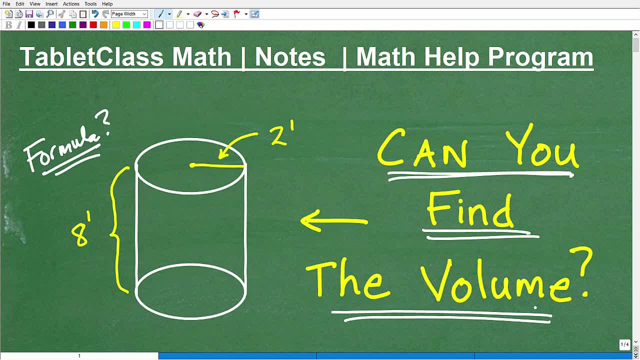 and do so because I'm going to get into the solution here in just one second. But first let me quickly introduce myself. My name is John. I'm the founder of Tablet Class Math. I'm also a middle and high school math teacher, And over several years I've constructed what I like to. 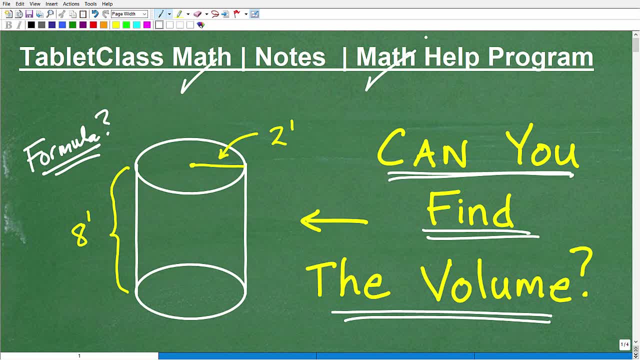 believe is one of the best online math help programs there is. Of course, I'll let you be the judge of that. If you're interested, you can check out my math help program by following the link in the description of this video. But basically I have 100 plus different math courses, ranging from: 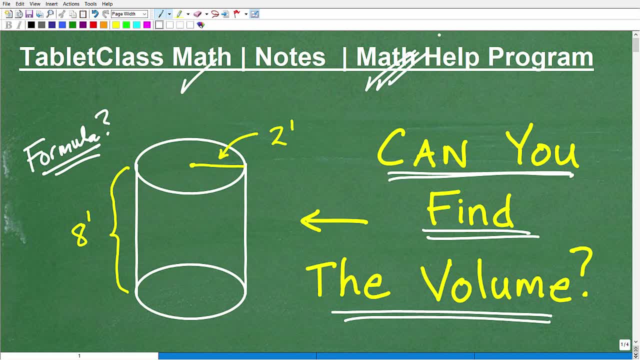 pre-algebra- Algebra 1,. Geometry- Algebra 2.. I'm going to be launching pre-calculus here in about a week, Really excited about that. But I also have many, many courses in the area of test preparation. So if you're studying for the GED, SAT, 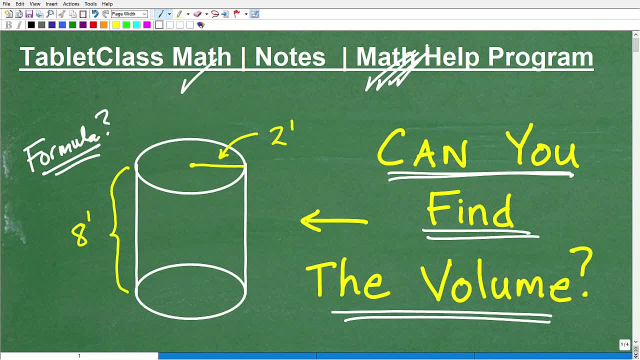 ACT, GRE, GMAT, ASVAB, CLEP exam, ACCUPLACER, ALEX, maybe a teacher certification exam, and many others that involve math and almost all these type of exams that people have to take. there's some sort of math section on them. Okay, if you don't do well in the math section. 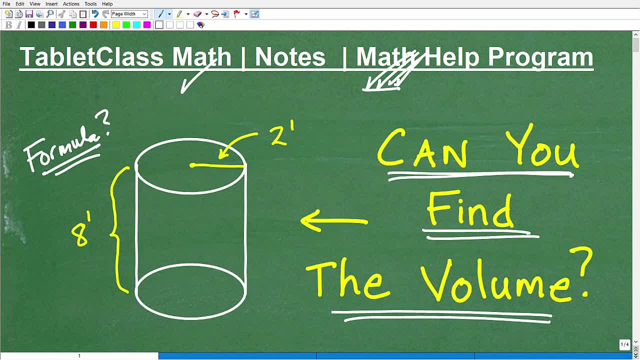 you don't do well on these exams. So believe me when I tell you whether you're going to college, vocational school, somewhere along your time, somewhere on your path in your career, sort of professional exam that has math on it. Okay, I can help you out. Just go to my website. 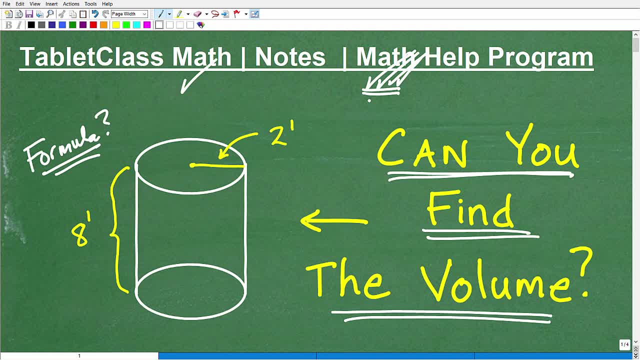 If I don't have your exam, drop me a line and I'll help you out the best I can. I also do a lot with homeschoolers, So if you homeschool, I have a great homeschool learning system And then obviously, help those of you that are just having a tough time in your current math courses. Now, if you, 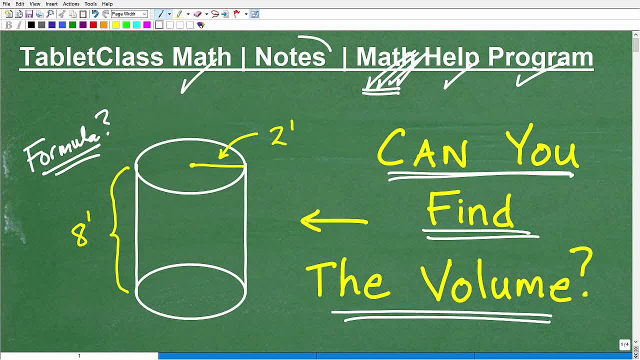 are truly serious about wanting to be great in mathematics, well then, you got to be great at taking math notes. Okay, this isn't, it's a simple concept, but it requires you to put in the math, the work every day. But if you do this, you're going to do very well, right? So, over decades of 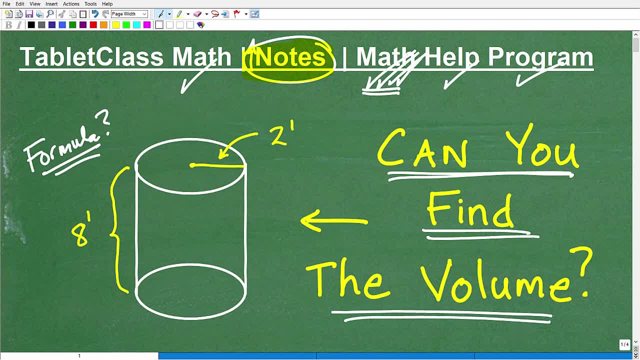 teaching math. this has been like the one thing that I can kind of, you know, point to be like: okay, when I see students taking great notes, I'm like they're going to do well, And the reverse is true When those students were like me way back in 1985, 86,, 87,, 83, or maybe the whole 80s. 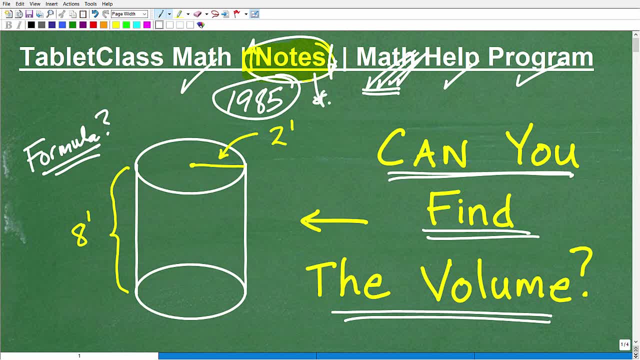 maybe even the 70s. What did I do? I was taking notes, but they had nothing to do with math and math class. They were like, Hey, are we going to that party? And then I went to get grades like this. So if you have a difficult, 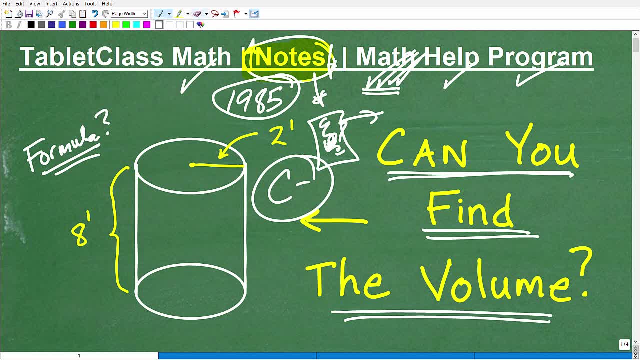 time in your current math courses, you're going to ask yourself: are you putting in the work Because you can watch all the little videos like this in the world, but you're not going to retain this stuff, All right. So you're here to learn math. I'm here to also emphasize how to truly 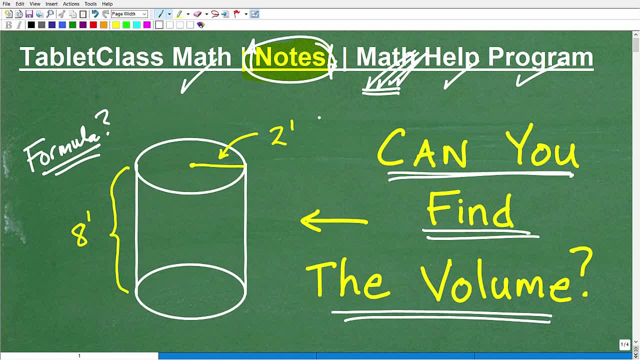 you know, be great at math Now. in the meantime, you still need something to study from, So you can use my math notes. Those would include pre-authors, algebra, algebra one, geometry, algebra two and trigonometry. You can find the links to those. 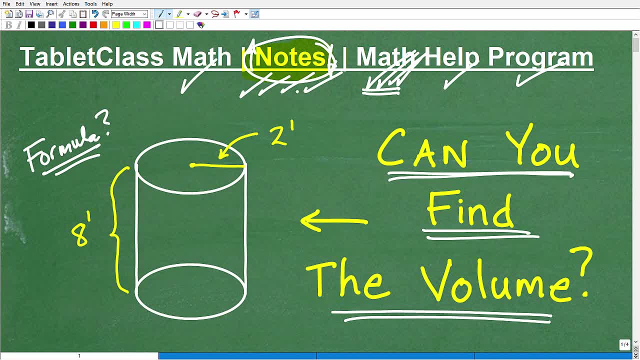 notes in the description of this video as well. Okay, So let's get to this problem. We had a lovely cylinder here, And so let me give. I'm going to tell you what the volume here is. Okay, But I'm going to give you kind of a the formula for the volume. I'm going to give you a little. 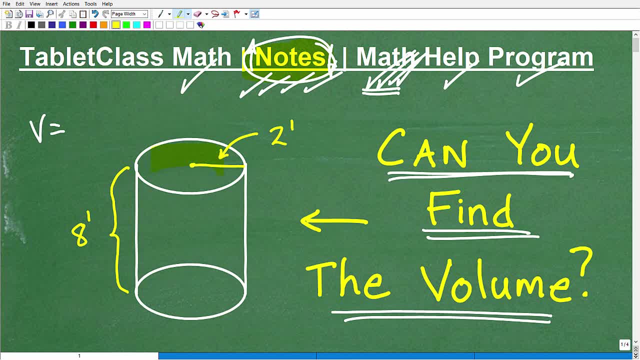 bit of. I'm going to do this kind of like as a hint. Okay, So the volume is going to be the area of this circle. All right, So we'll call that like the base times the height. Okay, So, if you can do, 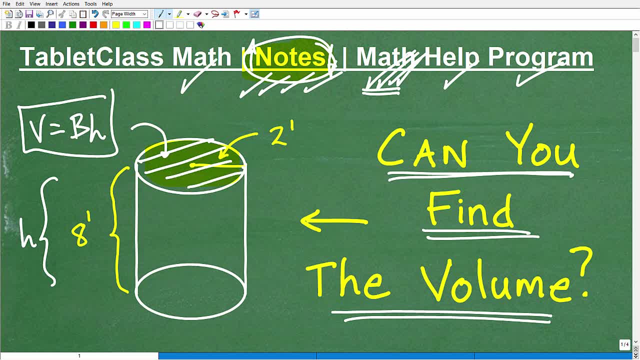 this: if you can find the volume of circle. So I'm asking right now: can you find the- I'm not the volume, sorry, the area? Okay, If you can find the area of the circle multiplied by the height, you will get the volume. Okay, So if you think you can do that, go ahead and do that now. 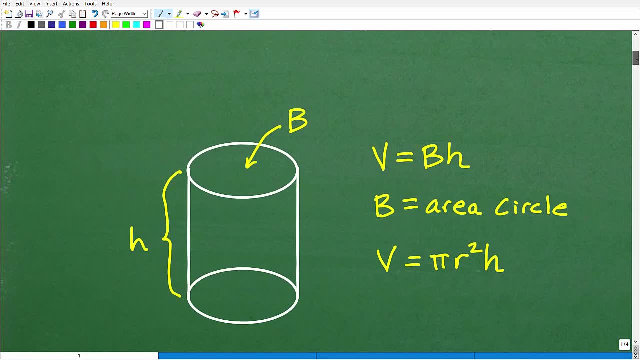 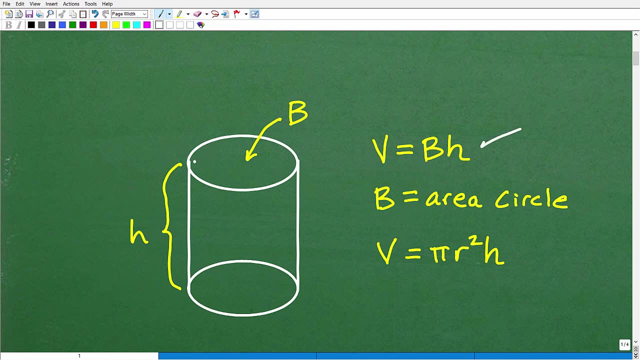 but let's get into the formula for the volume of a cylinder specifically. So again, as I said, the volume is equal to the base, which would be the area of that base times the height of the cylinder. So the B here is the area of the circle. Area of a circle is what? Well, 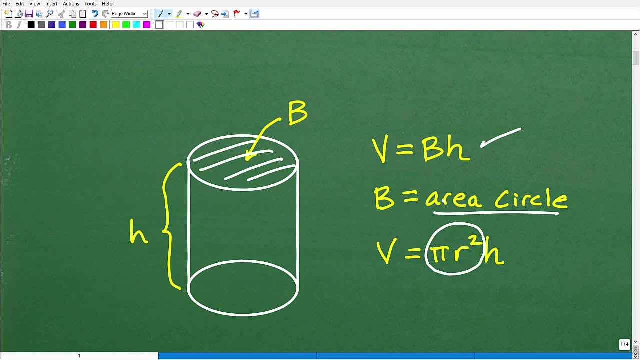 it is this right. here It's pi R squared. Okay, So really, this B is pi R squared, And what's R? that's the radius right That goes out from the center, out like. so Let me use a different color. 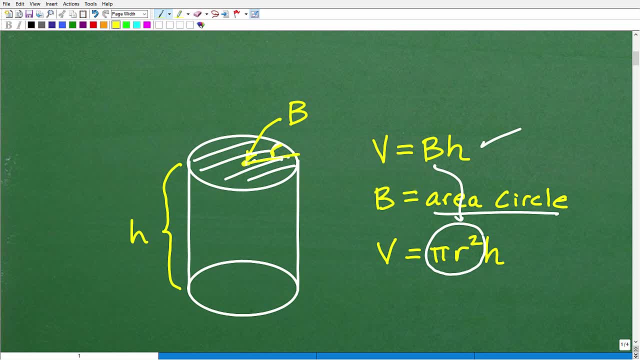 right From the center out to the edge of the circle is the radius. Let me multiply that by the height And you've got to be very mindful: We are dealing with volume. Okay, So real quick, because students, you know, they ignore these very important little details. All right, So let 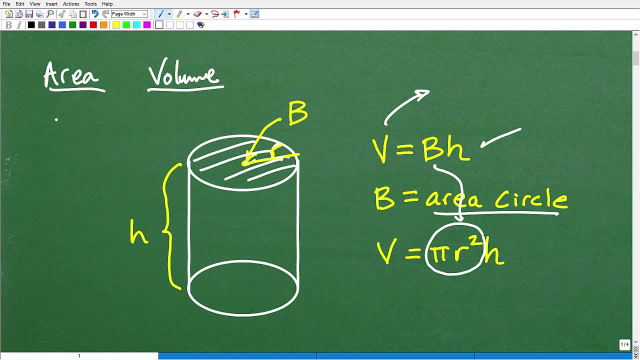 me just tell you real quick: So in area, your answers are going to be in units squared. So if we're dealing with feet and this particular problem, we're dealing with feet here. I think it's a eight and two, So area would be feet. 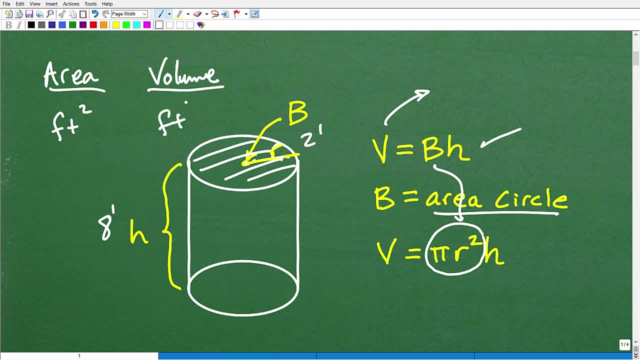 Squared, But volume is units cubed, So it's going to be feet cubed or centimeters cubed or millimeters cubed. whatever you're dealing with, Okay, Don't forget to use the proper units of measure, because most teachers- you know math and science teachers- will dock you points if you. 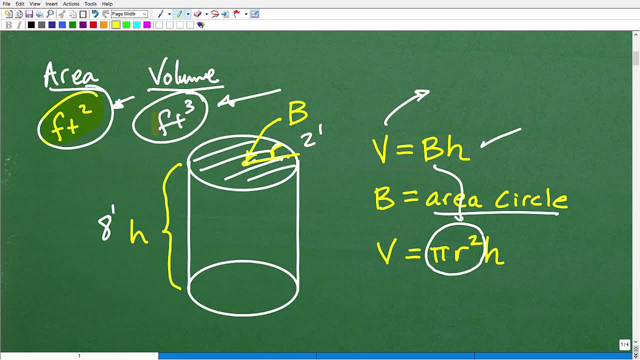 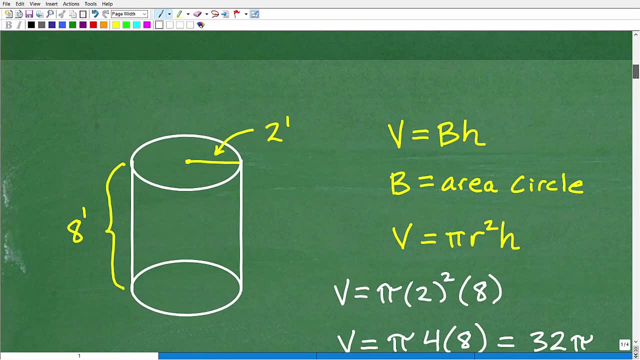 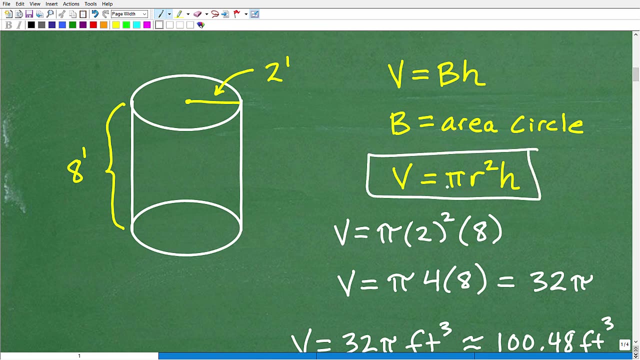 don't put in the proper units of measure. Okay, So pay attention to those guys at the end of your problem, All right. So let's get to the solution here And again. when you know the formula, you know this is not that difficult, All right, So here it is. Volume of a cylinder: pi r squared. 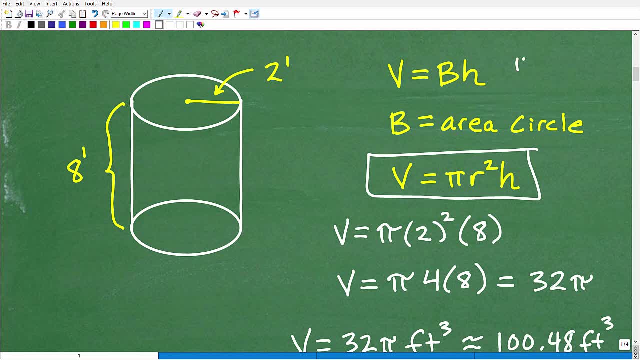 times h. So pi is what. Obviously it's the lovely number, approximately 3.14.. But we don't have to turn it into a decimal And I would just leave it as that symbol: pi. So our radius is two, Okay. 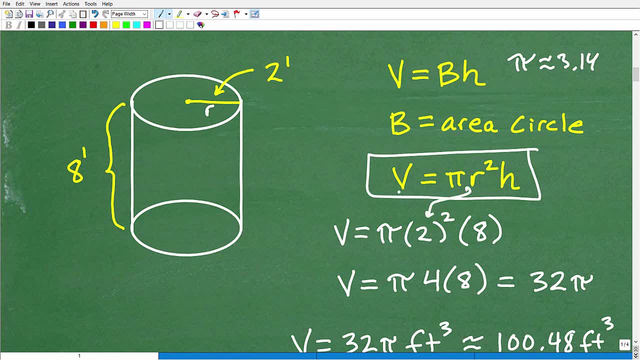 That's what r is equal to, So I'm going to plug that in Right. So then my height is h, So two squared is four. All right, I've got to do it. I'm doing this right here. Two squared is four. Remember PEMDAS? order of operations. all that good. 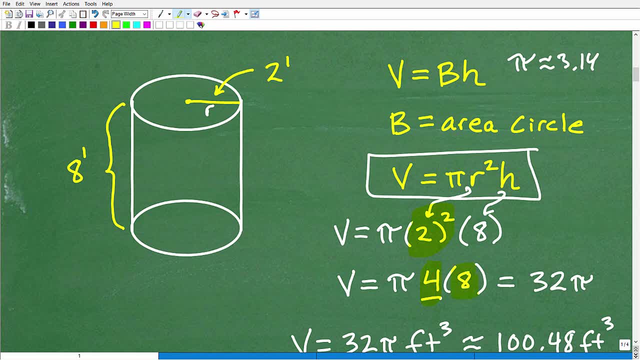 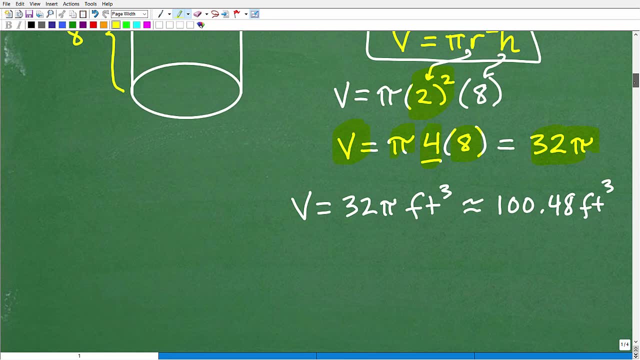 stuff. So I got to do the powers first. So I got four times eight, which of course is 32 times this pi. So my volume is equal to 32 pi. Okay, But remember units of measure, because this little 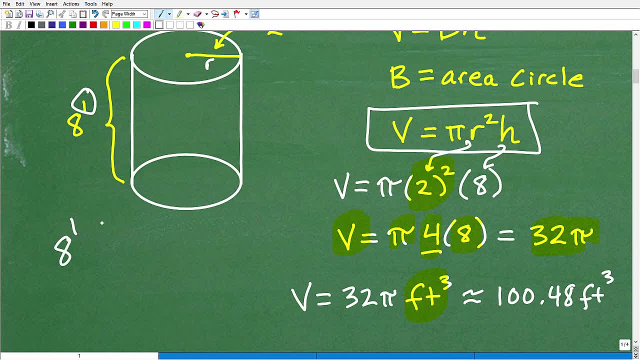 symbol right here, if you didn't know that little like this right here, this means feet, Okay, This means inches And this means feet, And you should be familiar with that. Okay, All right, So our answer. we can think of it in two. 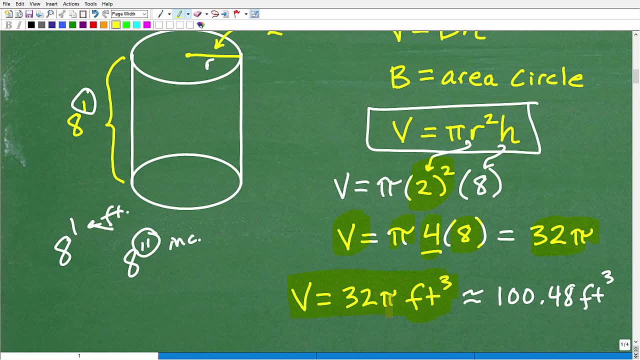 ways. Our exact, exact, precise answer is 32 pi feet cubed. So if I asked you for an exact answer, you would want to give me this. You would want to just keep that pi symbol in your answer. This is not a trivial little detail as well. Okay, Because this is exactly, precisely, 100% correct Now. 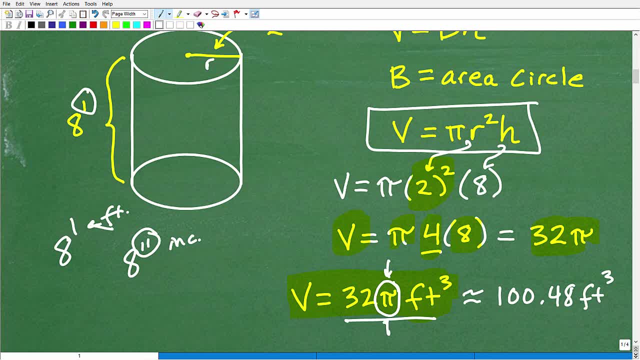 if I wanted a good decimal estimation then I have to go into my calculator and get a decimal for pi and take 32 and multiply it by 3.14,, yada, yada, yada And I would get about 100.48. 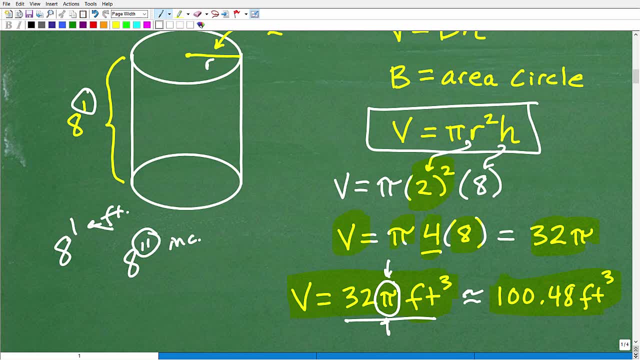 feet cubed, Okay, But again, this little squiggly mark right there means approximately: in math It's not equal to. So all these little details and stuff, they're important, Okay, Everything's important. So this is the exact answer And this is a nice decimal approximation. Again, notice that. 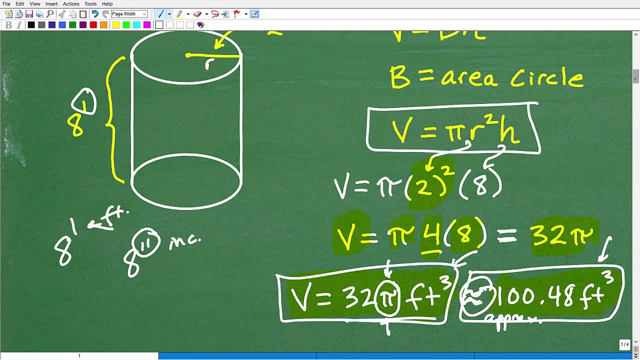 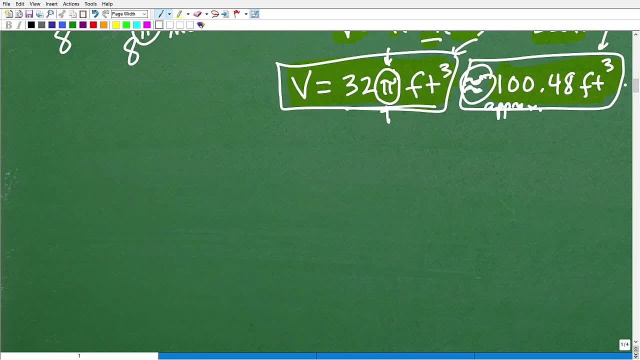 proper units of measure. But yeah, this is basic geometry and basic volume, you know, which would come into the category of learning area problems, volume problems, surface area problems and stuff that you absolutely need to know. Now, if you got this problem right, I'm going to give you a nice. 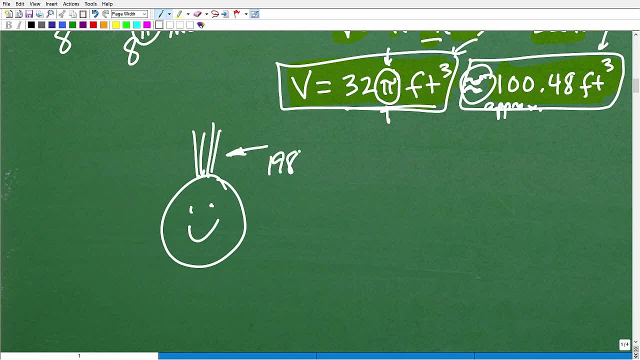 happy face with a good old fashioned 1983 Mohawk. Okay, So very, very good. I'll give you an A plus and I'll give you two stars. It wasn't the most difficult problem, But if you got this correct with the proper units of measure, that's excellent. Okay Now. 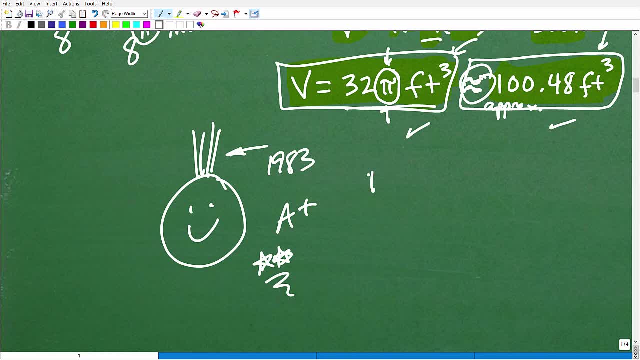 again, I'm going to encourage you to understand or get these formulas into your long-term memory. All right, There's a lot you're going to learn in math. that is just too much stuff. But you know again, working with basic shapes and figures, all this stuff you know, you should know, Okay. 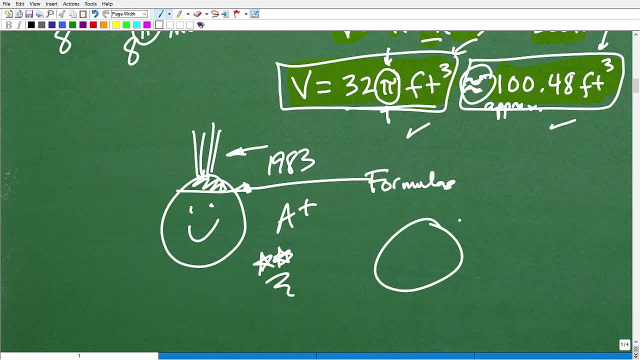 Certainly like the area of a circle and you know, area of a triangle, all that kind of stuff. But some surface area volume formulas come in handy And if you're taking excellent notes, okay, that's part of the process of learning and getting this stuff into your brain. That's why you want to do. 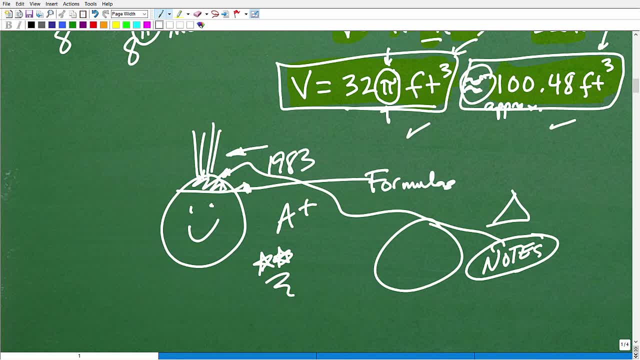 it. That's why it's not enough just to like: hey, look at your best friend's notes, Like, oh, they got great notes. No, it's the process We call that. you know, when you different learning styles. Okay, When you're listening, you're seeing and you're writing all this stuff. 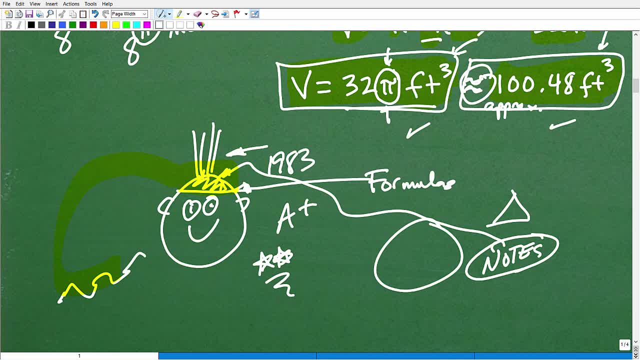 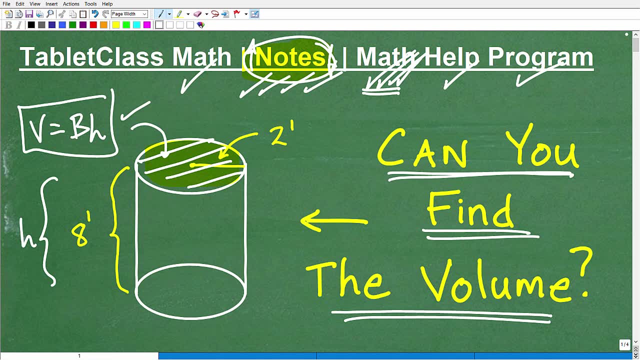 into your, you know rich, you know comprehension into your long-term memory. Okay, So you know again. I don't explain all this stuff precisely. in every one of my videos I tell you. this is the bottom line. The bottom line is that if you're looking for shortcuts, I haven't found them, And 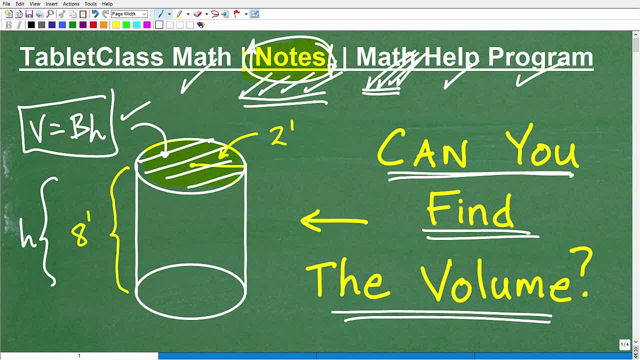 I've been doing this for decades and decades and decades. All right So, but if you're looking for the truth in terms of hey, yeah, you want to do good well in math, these are some of the things that you got to be working at, All right. But listen, you know, don't worry about it, You know. 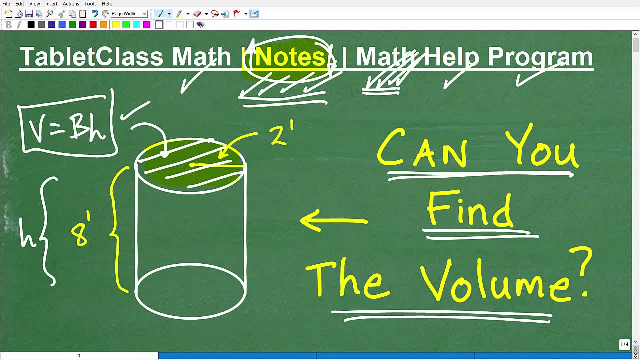 don't ignore basic volume problems, surface area problems, area problems. This is really, really important stuff and it shows up all the time. So a couple of suggestions. I have more of these type of videos in my pre-algebra algebra and my geometry playlist. Okay, You can practice, But 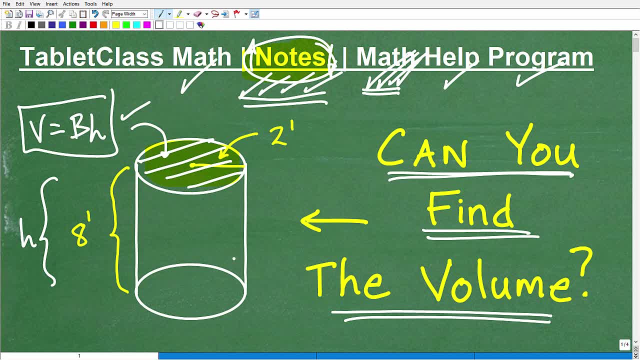 you know, depending on where you're at in terms of geometry. okay, I teach basic geometry in my pre-algebra course And then obviously, I teach it thoroughly in my geometry course, And it comes up again in other courses as well. All right, So that's it, Thank you. 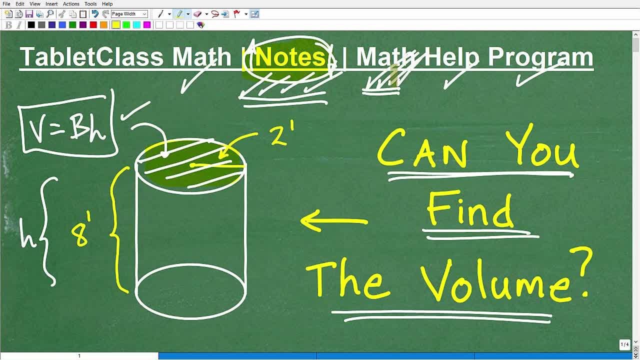 But those two courses you might be interested in. Of course that will be in my math help program. All right, If you liked this video to some degree, please consider smashing that like button and please consider subscribing. Been on YouTube for 10 plus years, have over 1,000 videos and I'm 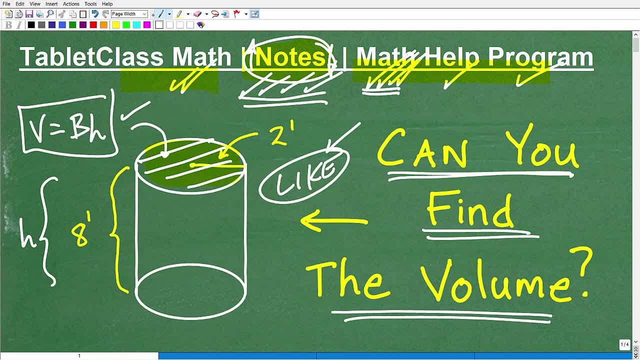 posting new content all the time, Okay? So, whether it's volume or, you know, algebra 2, logarithm, stuff, whatever the case is, you'll find a ton of videos on my channel: Basic to Advanced Math- all there for you, Okay. So, with that being said, I definitely wish you all the best in your